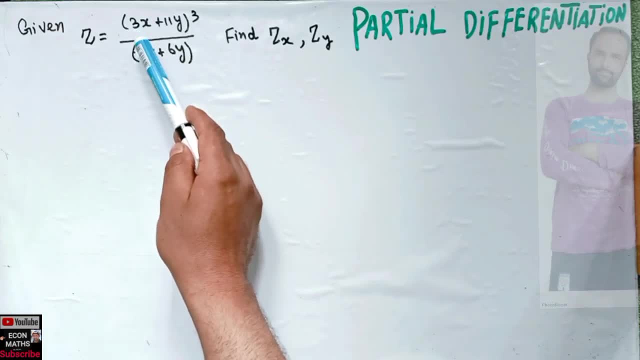 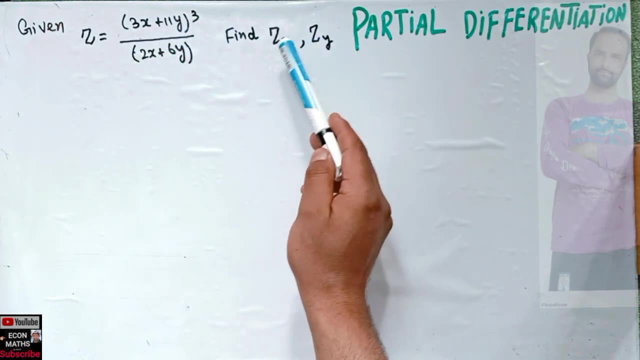 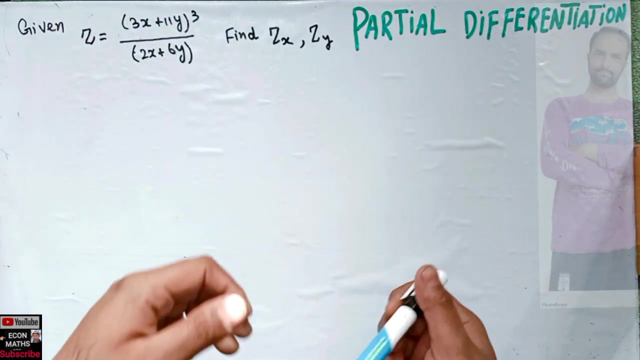 Given a multivariate function is: z is equal to 3x plus 11y. whole cube upon 2x plus 6y find zx and zy, where zx is the partial derivative of this function with respect to x and zy denotes the partial derivative of this function with respect to y. So how do we solve this very question? 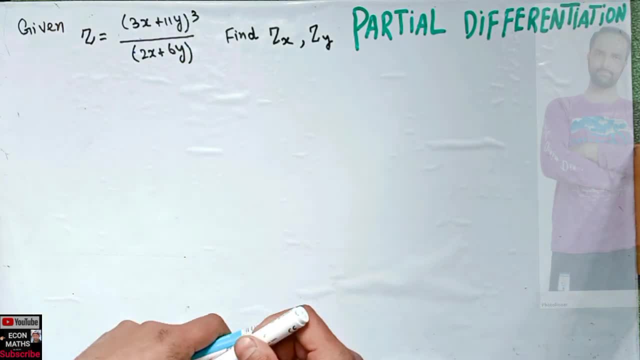 So in this case we have to apply quotient rule. okay, because we have here, you know, this numerator and denominator. the functions are in numerator and denominator. we can use the quotient rule here. What is exactly the quotient rule? Quotient rule is written like this: 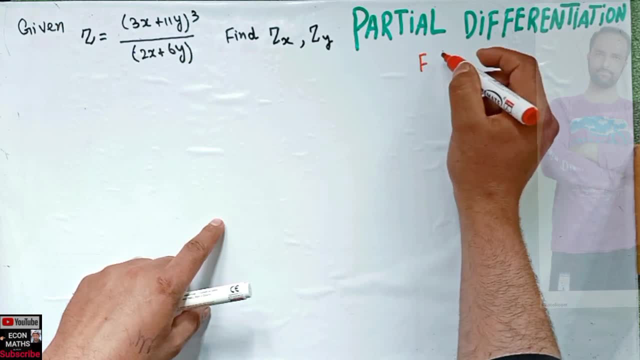 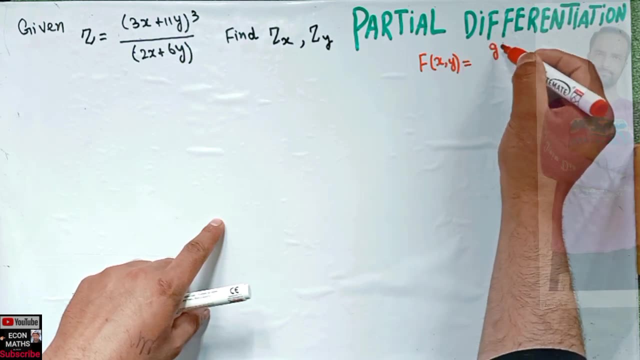 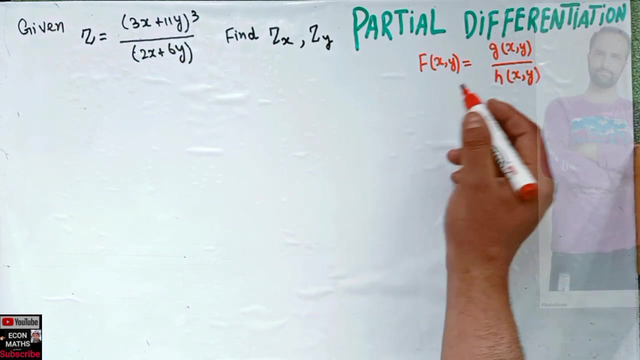 Let us say we have a function: f of xy is equal to g of xy upon h of xy. okay, So as this function is being given Now, taking partial derivative and using quotient rule, that means f subscript x. okay, This denotes partial derivative of this function, with respect. 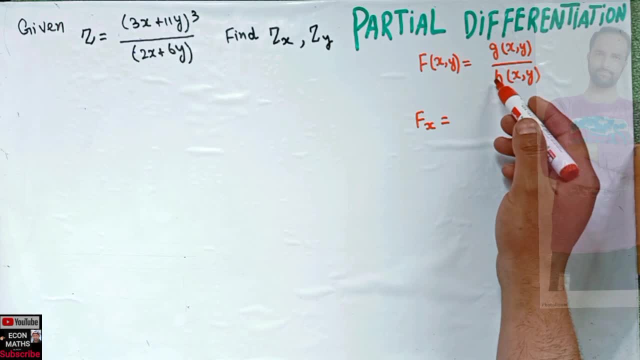 to x, and it is being given by simply: first we write this denominator function that is h xy, and take the partial derivative of this function that is g x, g xy. then we subtract and write this g xy as it is g xy, and then we take the partial derivative with respect to x again. 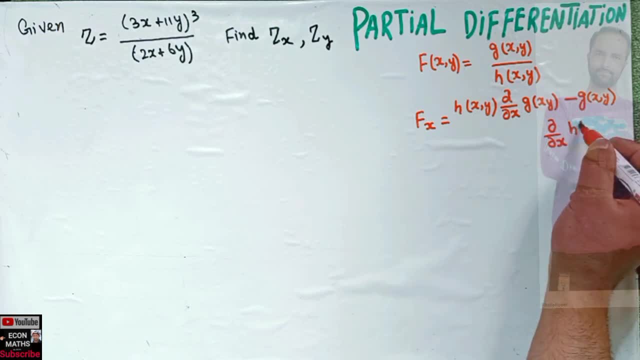 of this function, that is g, xy, And this is what we get. So this is h of xz and to this we divide by this h, x, y whole square. okay, This is the quotient rule that we need to apply. okay, So you will get this. 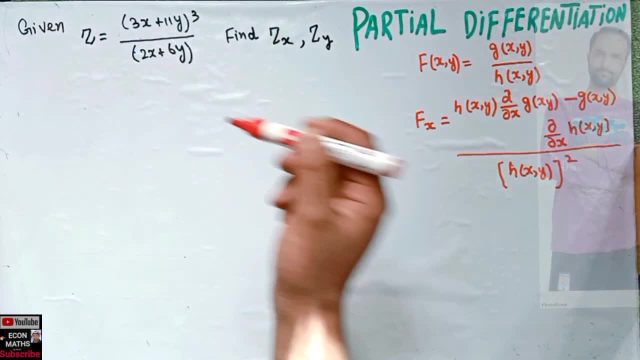 idea here Now, first finding z of x, So z subscript x means taking partial derivative of this function with respect to x. And then we have z of x, And here we do the first test, which is given by taking partial derivative of this function, by taking partial derivative of this function, by taking partial 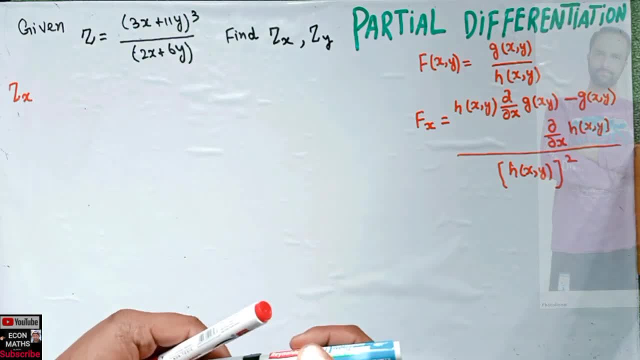 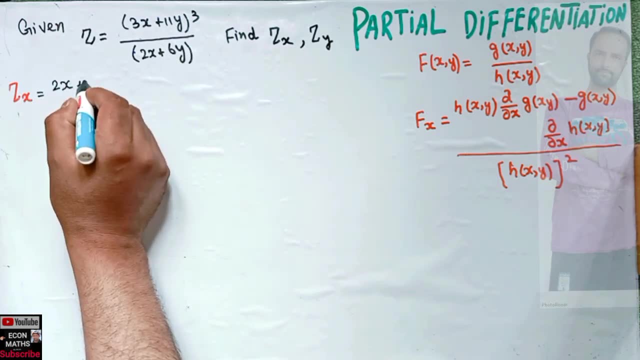 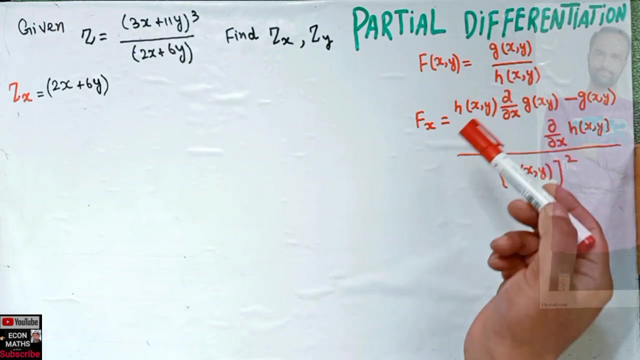 x, okay, so let's uh give some intuition here. so first we write this 2x plus 6y as it is, so i will write it as 2x plus 6y. okay, as i have explained here, first we write this h of x and then we 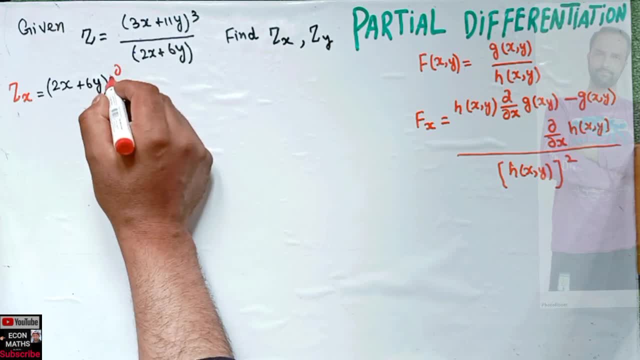 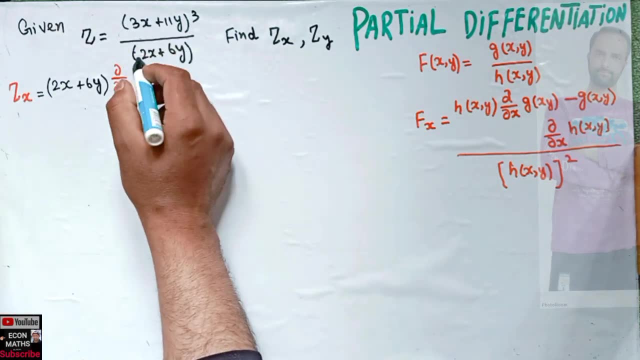 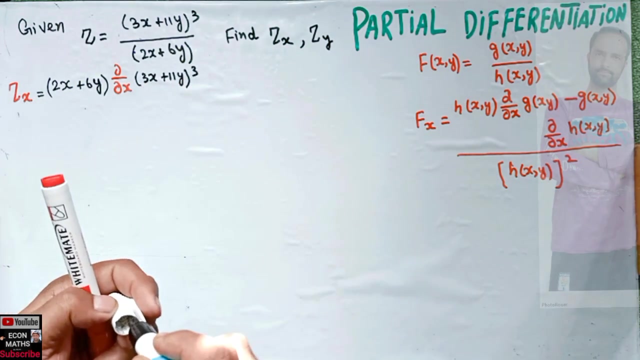 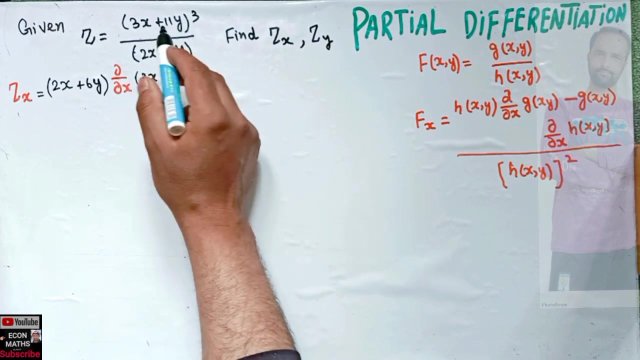 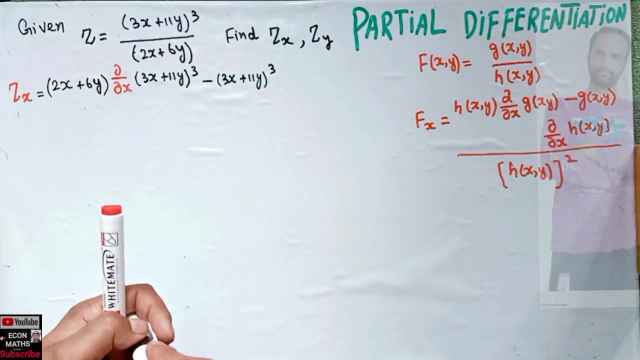 take the partial derivative of d upon dx of this function, that is 3x plus 11y, q minus. then we write this gx again. so in case, here our gx is 3x, 3x plus 11y cube. and again we take derivative d upon dx of now this function okay, 2x plus 6y. 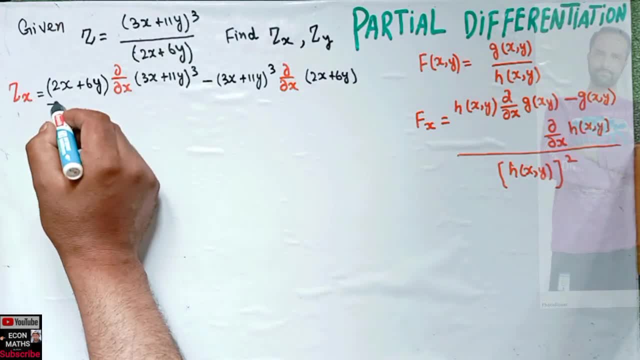 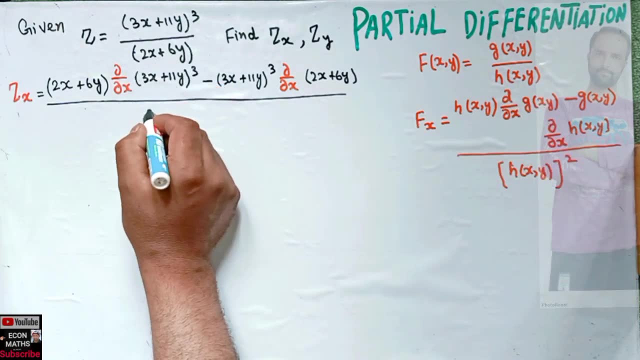 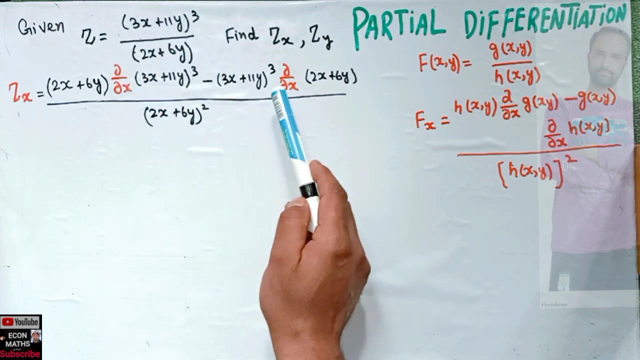 and we divide it by h x- y whole square. so this is our h x y. so we have 2x, 2x plus 6y, whole square. okay, very simple enough. that is. first, we write this function and take derivative of this function. minus, we write this function and take derivative of this function. 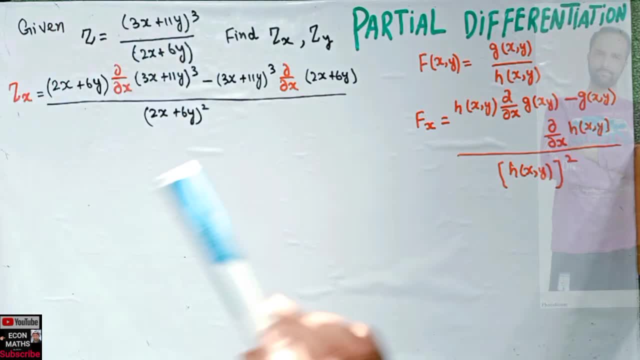 and whole divided by this function. but it is square. okay, simple stuff here. now doing our differentiation: here we have 2x, as it is 2x plus 6y, now derivative of this function, d upon dx. i will write it here to make the things easier. now: d upon dx of. 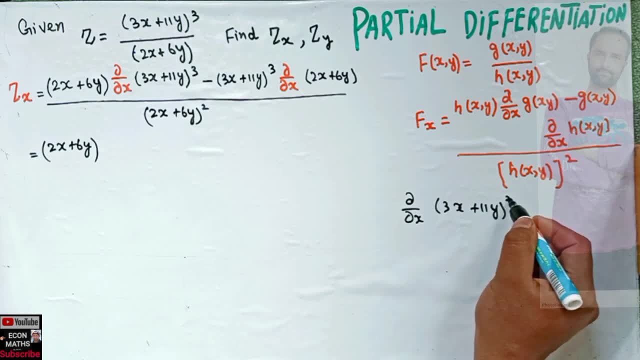 3x plus 11y cube will mean that we need to differentiate this function with respect to x. so first this will become this: exponent becomes coefficient, as i have explained it so many times, plus 11 y square. now 3 minus 1 is 2, okay, and exponent is subtracted by 1. then we need to multiply and 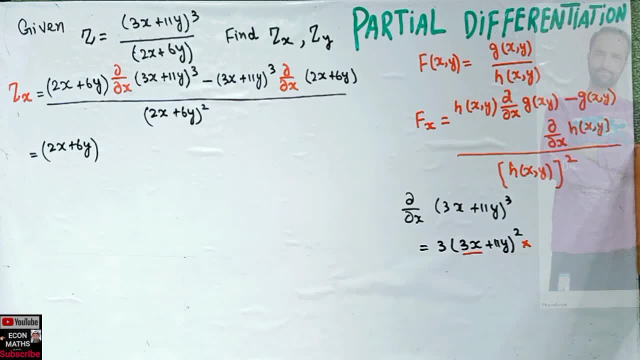 since we have 3x again in the brackets, we need to take the derivative of this d upon d x of 3x. okay, so we will get 3, 3x plus 11 y square, and internally the derivative of 3x is 2x- 2x. so we will get 3x, 3x plus 11 y square, and internally the derivative of 3x is 0.. 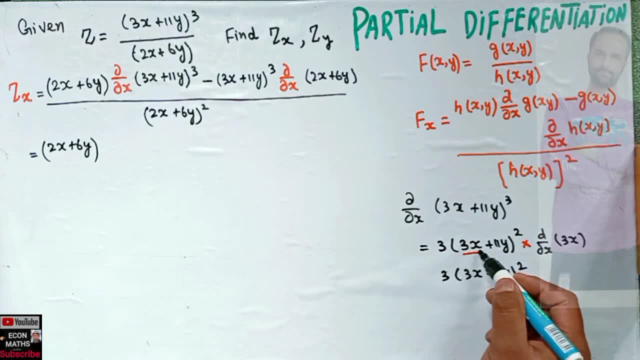 square, and internally the derivative of 3x is 0.. is only 3 here, so derivative of x is 1, so we are left with 3 only. okay, so this will become 9, 3x plus 11 y square. okay, so the derivative of this stuff, this stuff, will become this. okay, i will. 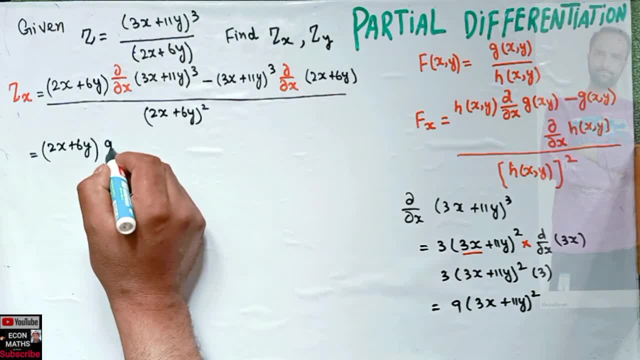 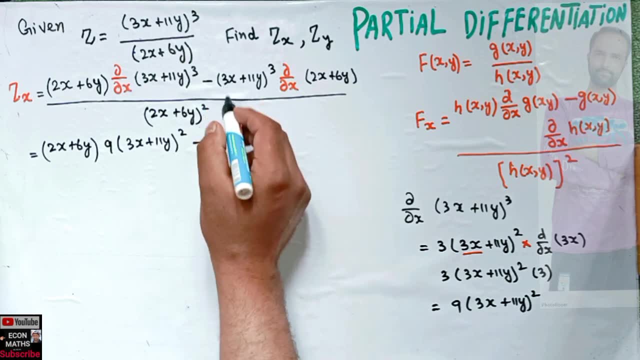 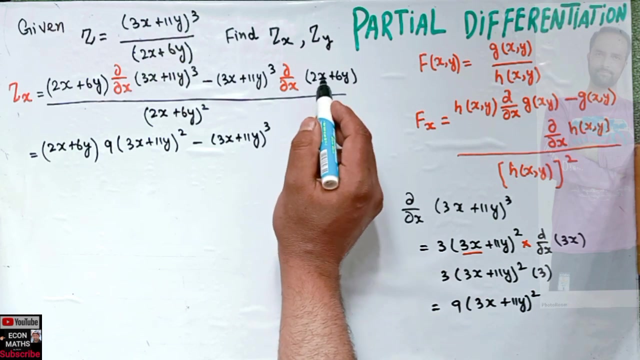 explain it here, so let me write it here. we have 9, 3x plus 11, y square minus. then we have this function, 3x plus 11, y cube, and derivative of this function with respect to x. since only one term is here, x, so derivative of x is 1, so we are left with 2 only. so we have 2 here. okay, so i will write here. 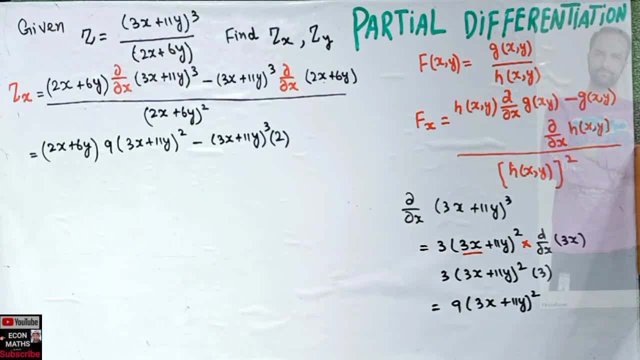 2. okay, and derivative of constant is of course 0, so let's cut it short here. then we have 2x plus 6y. okay, very simple enough. now what will we do here? we will factor out if there is any term like so. here we can see 3x plus 11 y, 3x plus 11 y- here it is cube, here it is square. so we can. 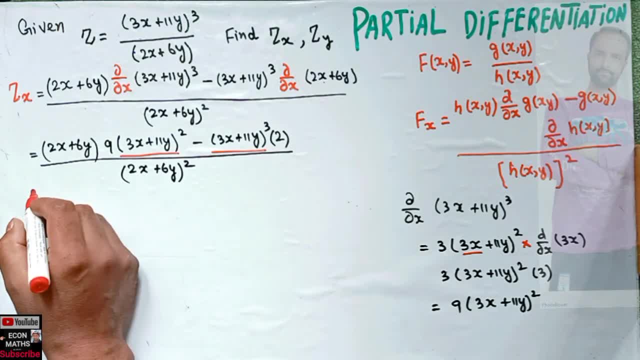 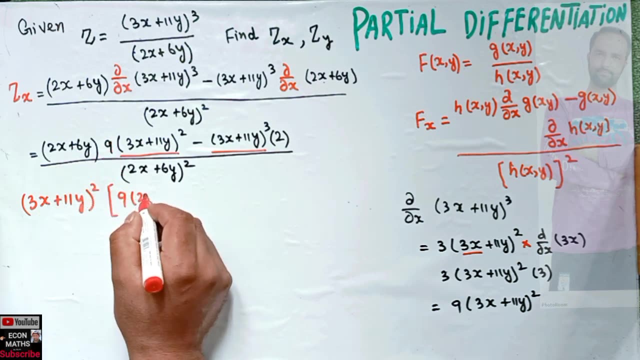 take square terms common, so i can write it like this: 3x plus 11 y. i have taken it out later. okay, clearly seen here. ok, now, here is left. there is no name. here'll rotate that square, so here's it here, seu u. ok, now what we are called. this is two Plan. we are called: 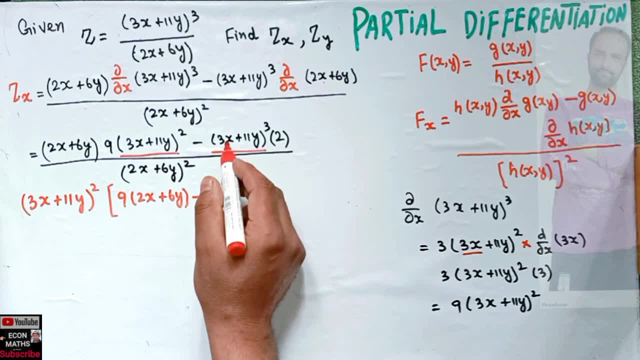 lambda. okay, in case we work out why lambda it? our function classic module: okay, and it seems we are left with 2 here, so it should be a two or less than the s, and so we have taken 1 cube here, 2x, and that's it. so here we have. we are left with 1, so hereメ. 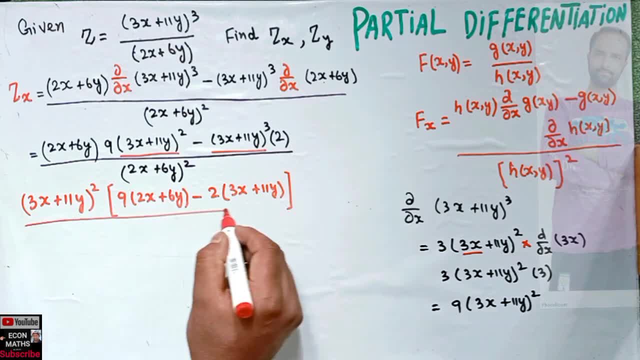 o, ну, okay, then what we are being left? we are being left with 9liness. okay, so we have a plus six y talisman. okay, then of course, we have minus this two, 3x plus eleven y. oops, then will be like this: so we have 2x plus 6y square here. okay, now we have 3x plus 11y. 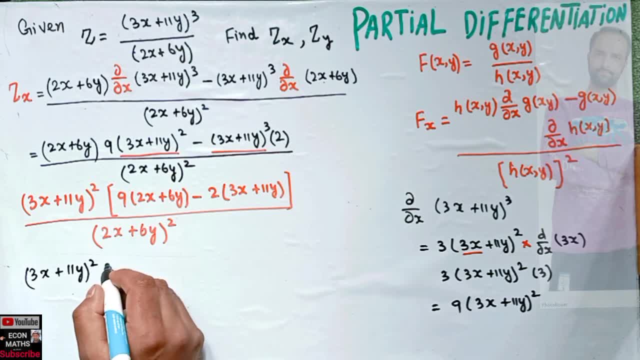 square doing some calculation here. so 9 to the 18, 18 X, 9, 6 R, 9, 6 R, 9, 6 R. go to another. so this is 54, 54 Y. okay, minus 2, 3's are 6x, minus 2 11's are, so Y and we. 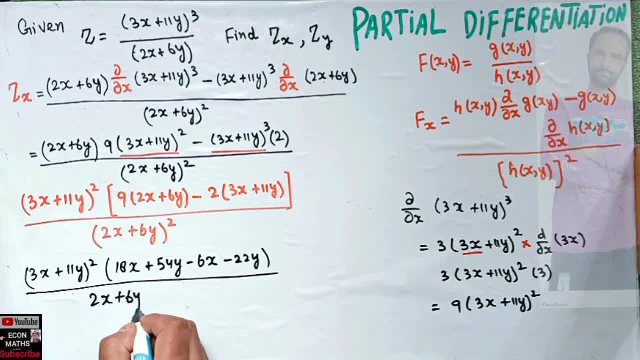 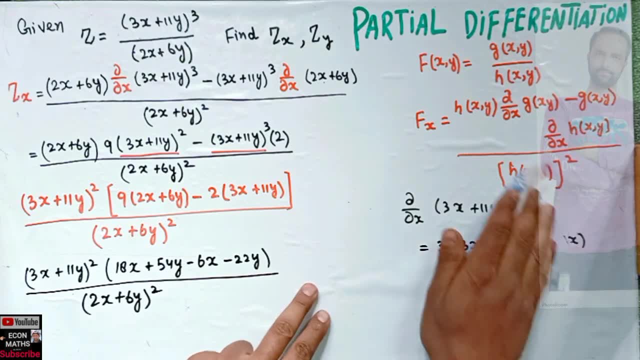 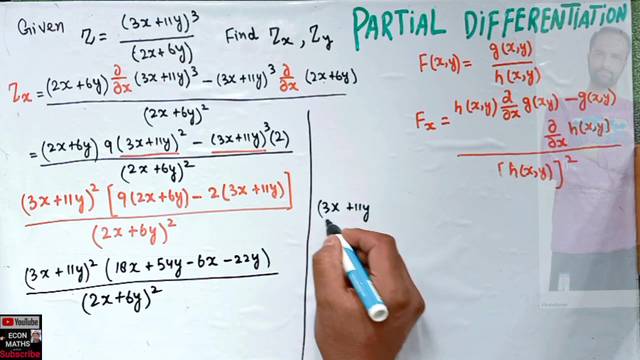 divided by this: 2x plus six YY. okay, let me wrap this out. okay, so we have here 3 X plus 11 Y S square, now 18 minus 6. is other онаح лучше here? sure, sure, I shall be. so this is to Alex. okay, to a like this one's on wall of the. 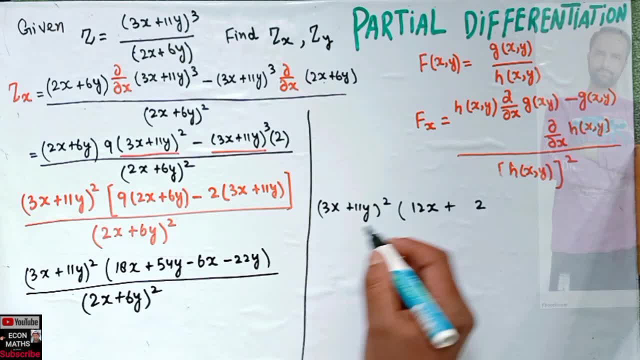 door and is it is, we have to hear parts and it's the 332 Y. okay, I just subtract with the like terms. I will subtract 6 X from 11 X and 22 Y from 54 Y and I got this very stuff. then we have 2 X plus 6 y square. okay, can we do some further? 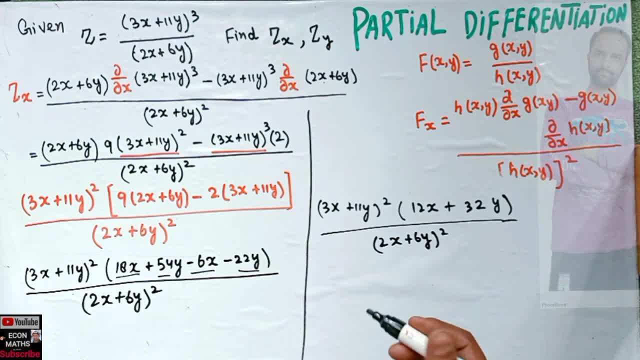 simplification, simplification here let's try to see. so we have 3 X plus 11 Y square. let's take 4 common here. so we have 4. we are left with 3 X plus 4 a 32, So we have 8y. upon here we can take 2 square common, okay. 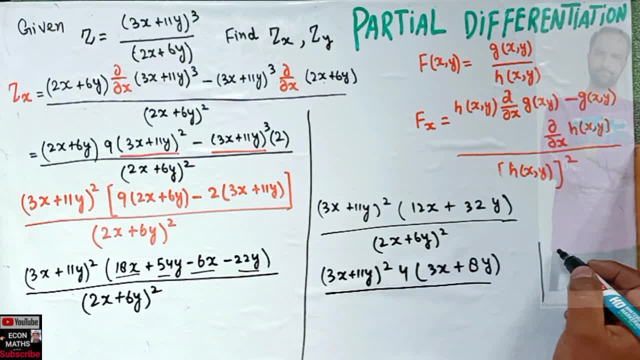 So let's explain it here. If we have this very stuff- 2x plus 6y- square, I can write it like this: 2x plus 3y- okay, square. like this: Then I can give this square to each of these terms: 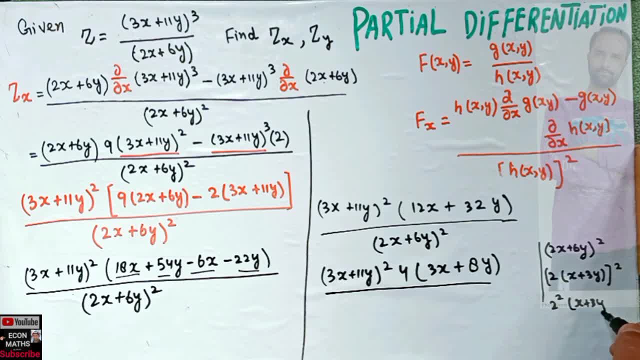 So we have 2 square and x plus 3y square, So this is 4x plus 3y square. okay, This stuff becomes this, so I can write here: 4x plus 3y square, 4, and 4 gets cancelled. 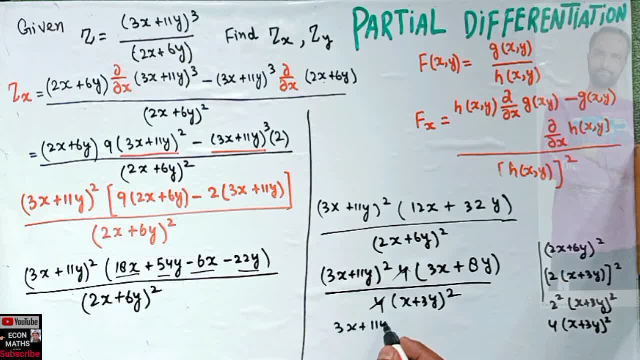 So we are left with 3x plus 11y. Then we have 3x plus 8y- I hope I am making the calculation right here- And we have x plus 3y square. okay, So this was our zx, okay. 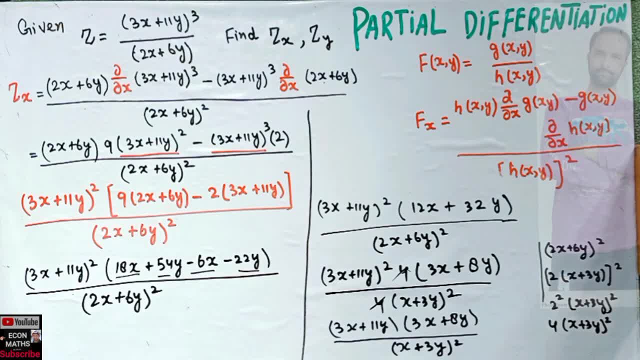 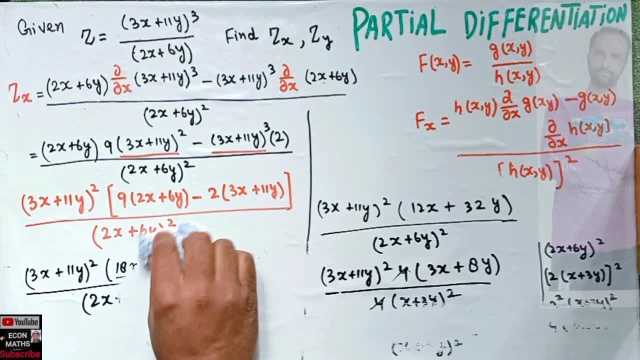 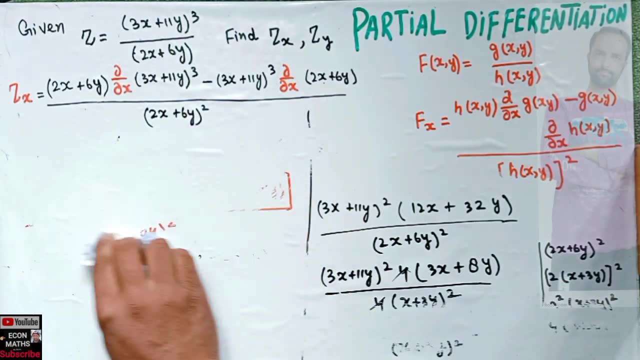 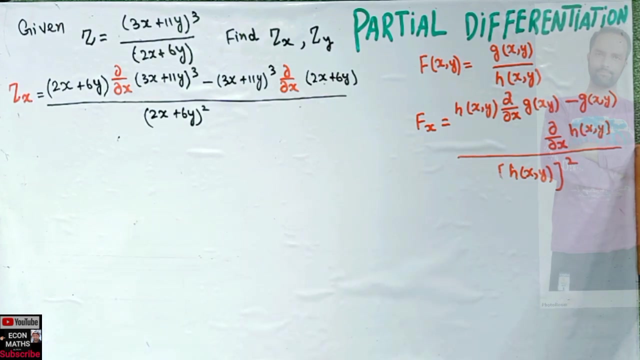 So similarly, we can find out zy. okay, Let me try to find out zy also. For that I have to rub this out, okay, So So let us write it here. Now we need to find out z. subscript y. 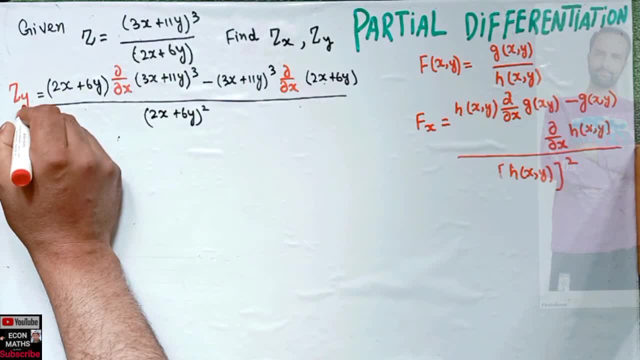 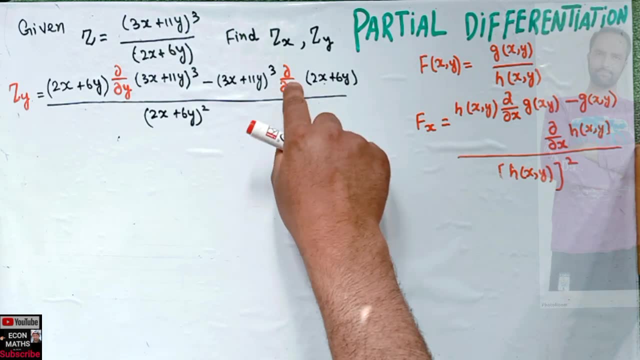 That means partial derivative of this function with respect to y. okay, So this will remain the same, but we have to take partial derivative with respect to y this time. okay, So we have y here. we have y here. okay, simple stuff. how do we do use the? 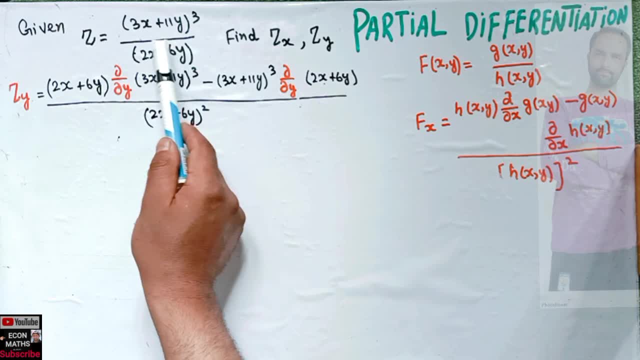 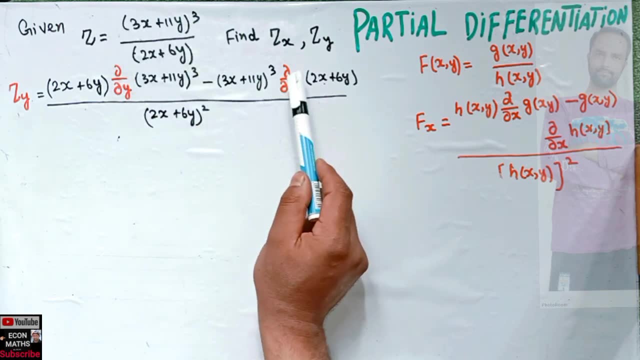 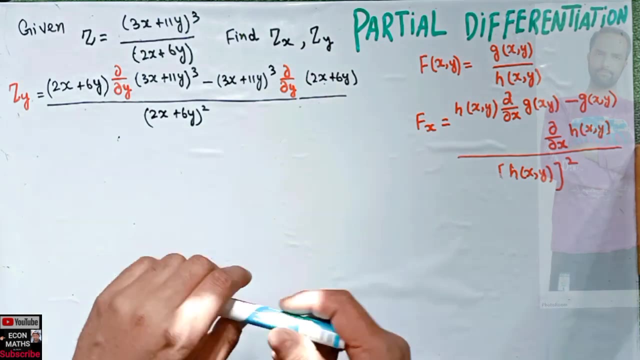 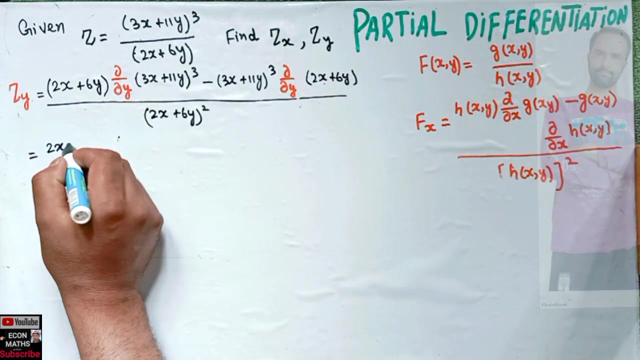 quotient rule. first we write the numerator- sorry, denominator, this function, and take derivative of numerator minus numerator function. the derivative of denominator function whole divided by denominator function square. okay, simple stuff now using the same as stuff here. so we have 2x, 2x plus 6y. 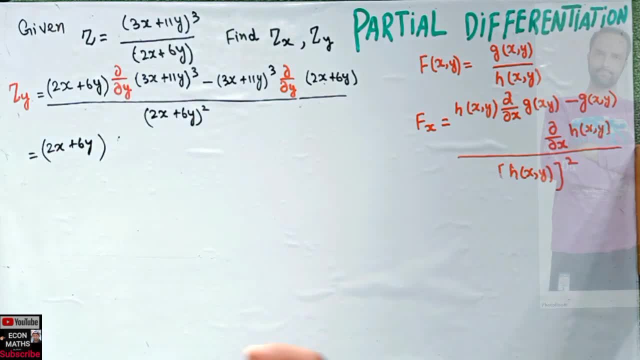 as it is now derivative of this function, as I have explained it here. so first we need to take the power function rule. that means 3, 3x plus 11, y, 3 minus 1 is 2, so this becomes square. so first we we. 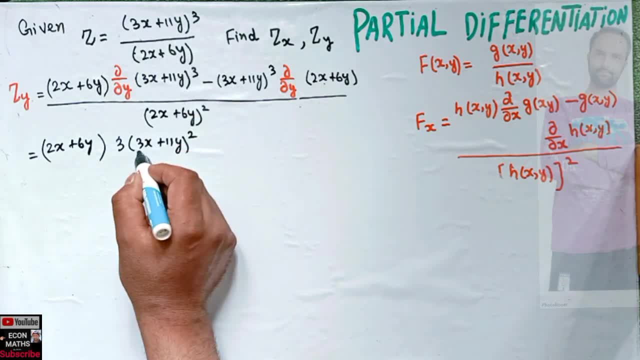 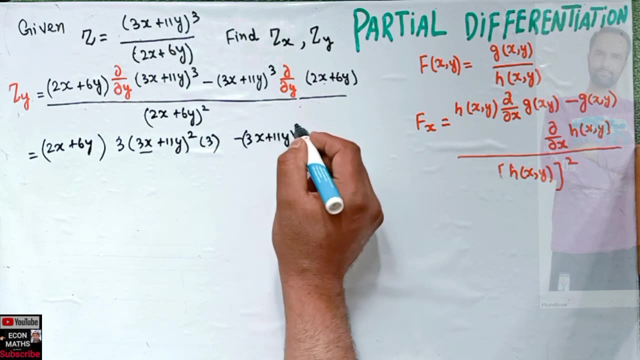 use the power function rule. then we have to internally differentiate with respect to x. so derivative of 3x is 3, so we multiply it by 3. okay, then we have minus 3x plus 11 y. cube derivative of 6y will be 6, because no y is involved in. 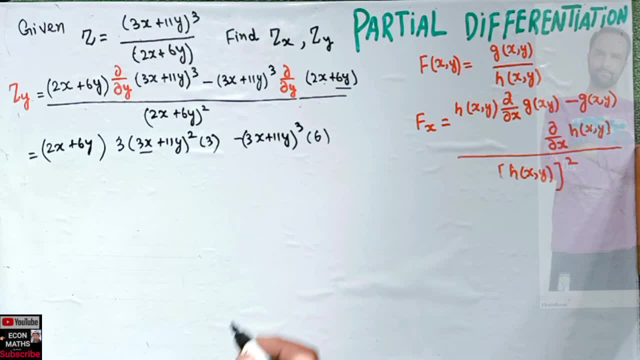 this term, its derivative will be 0, so we are left with 6 only. okay, sorry, we have two plus 6. we are taking the derivative with respect to y. so here we are. we have to internally differentiate with respect to why you you derivative y is 1, so we are left with 11. okay, it was an horrendous. 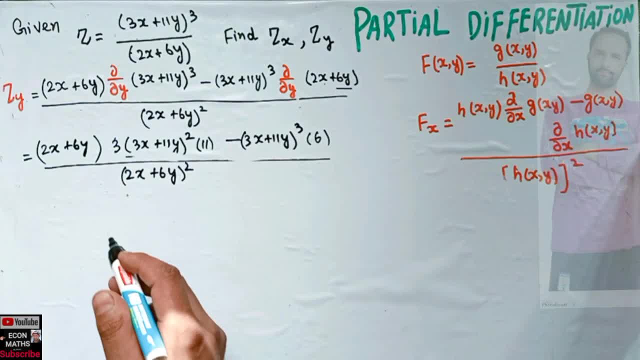 mistake here. Now we can do one thing here We have 11, threes are 33.. Okay, So we can first take this 3x plus 11y square common, Okay. Then we have 11, threes are 33.. 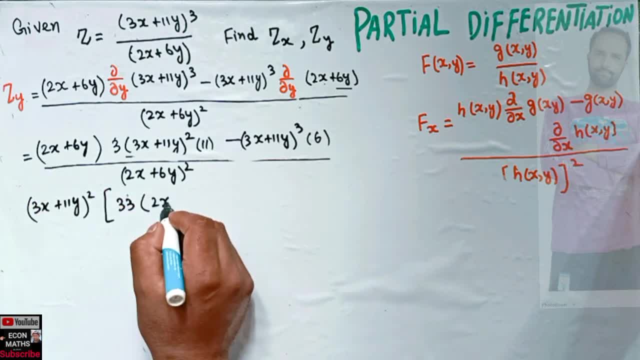 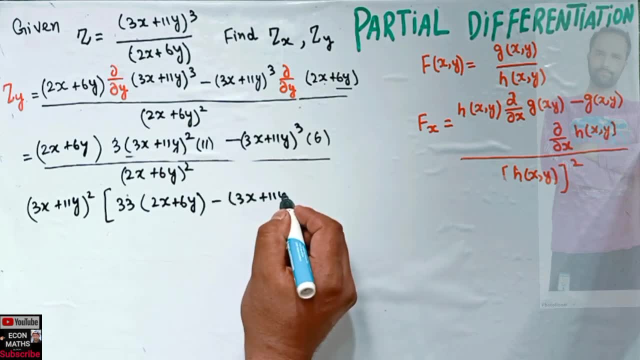 Okay, We have this term 2x plus 6y minus 3x plus 11y, So let's write this 6 here, Okay, Divided by this term 2x plus 6y whole square. Okay, Now we have 3x plus 11y whole square. 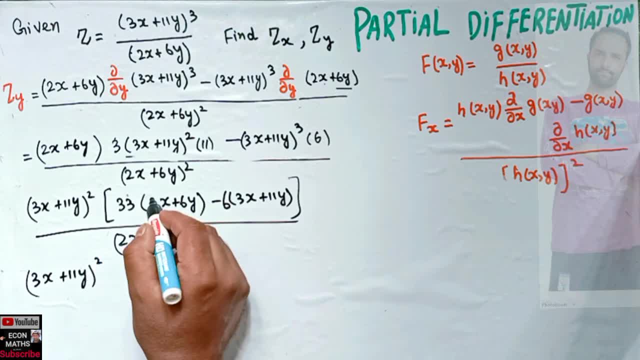 Okay, I am Okay. This is 2x here. So what we are being left here? Let us take 3 common here. now. Okay, If I take 3 common, we are left with 11.. 2x plus 6y minus 311 are 33.. 3x plus 11y- Okay, I have taken 3 common. 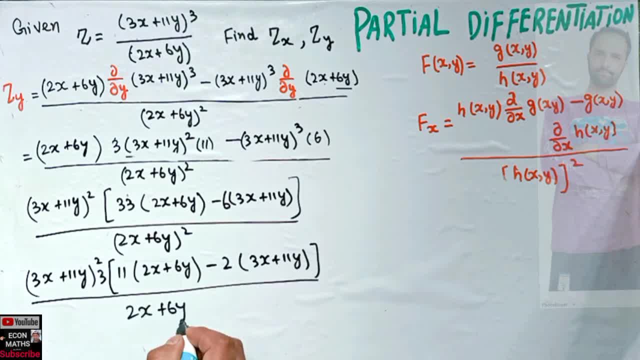 Okay, So we have 3x plus 11y whole divided by 2x plus 6y square. Okay, I hope the calculation is going right. At times there can happen some horrendous mistakes in my videos, obviously. So let's write this 3 here. We have 3x plus 11y square. I have just written this 3 here because we know multiplication is commutative. 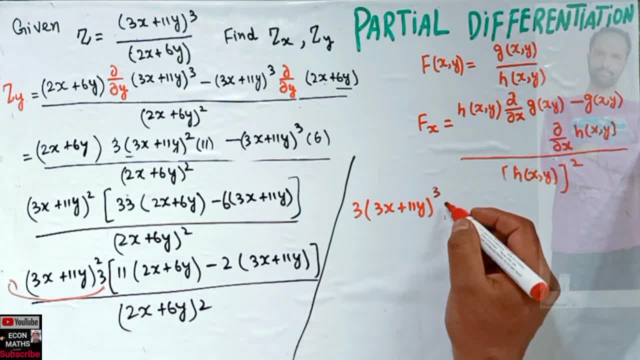 Okay, So the cube is here Now. 11 twos are 22.. 22x plus 66y minus 6x minus 22y 22y. Okay, I have just multiplied this 11 to each of these terms and this 2 to each of these terms, So 11 twos are 22.. 11 sixes are 66.. 2 threes are 6.. 2- 11 threes are 6.. 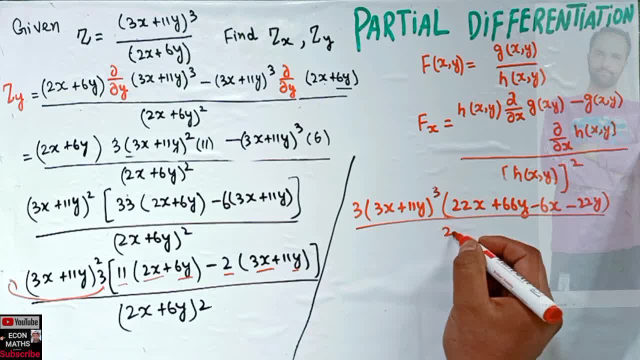 These are 22 whole. divided by this, 2x plus 6y square, Okay, So we have 3x plus 11y cube. Now 22 minus 6 comes out to be 16x. Okay. Now, short and large is 2.. 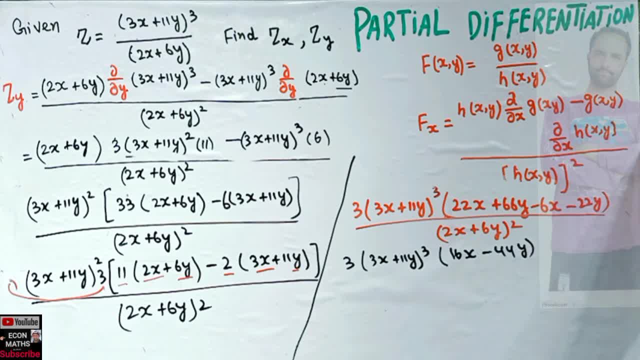 44y divided by 2x plus 6y, whole square. Okay, Now we can write it like this: 3. We have 3x plus 11y. It is square here. Okay, I am doing again the mistakes.